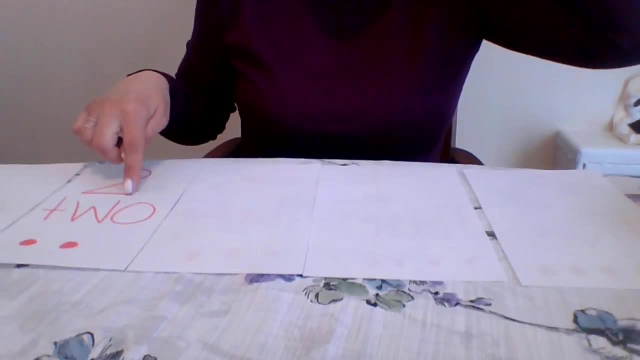 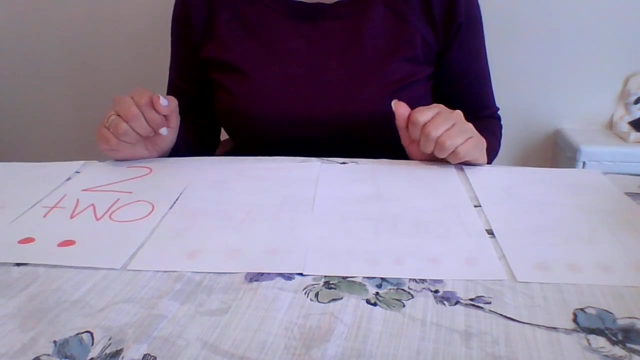 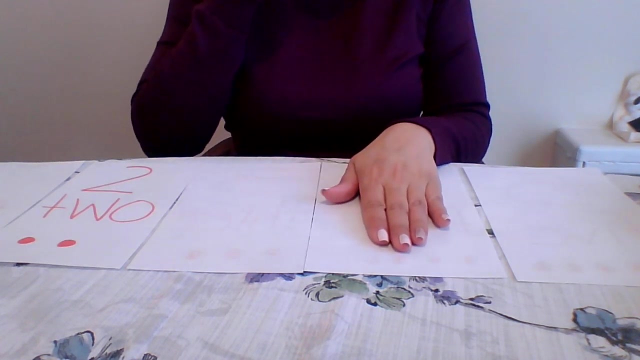 1, 2.. So we're going to leave this card facing this way, This card facing up. Okay, We're going to choose another card. Okay, I'm going to choose this one And make sure you use your x-ray vision glasses to tell us what's under this card. 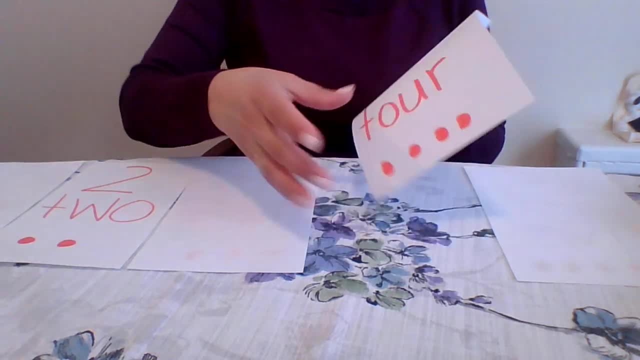 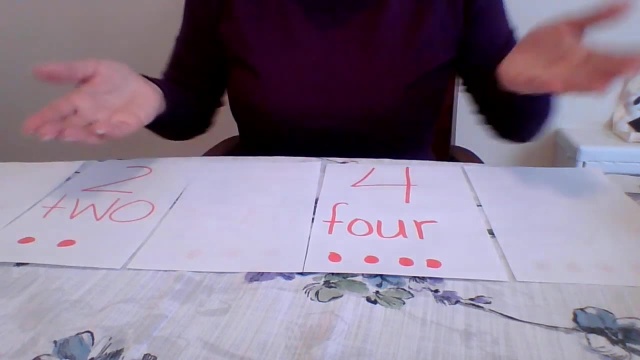 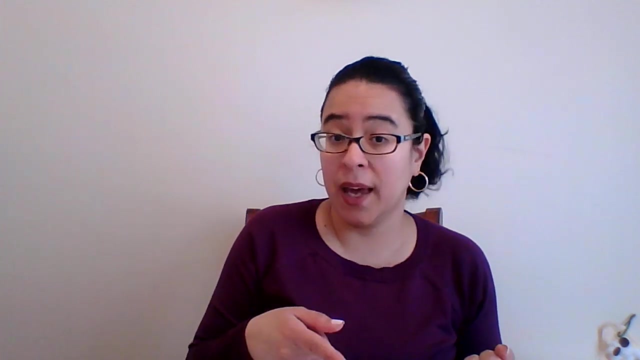 Let's see Who can tell us 4? Yes, it's 4.. The number 4 is under this card, Okay. So how did you know it was the number 4? Because? okay, because you knew that 1 starts here, right. 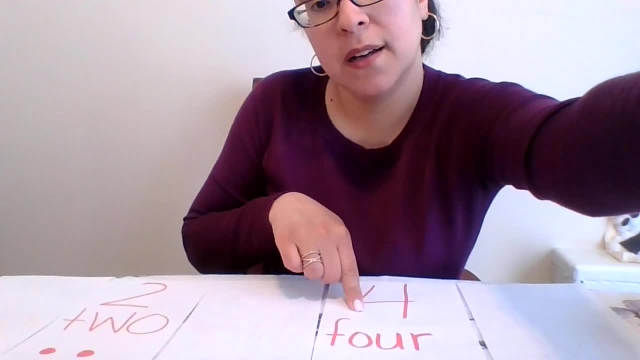 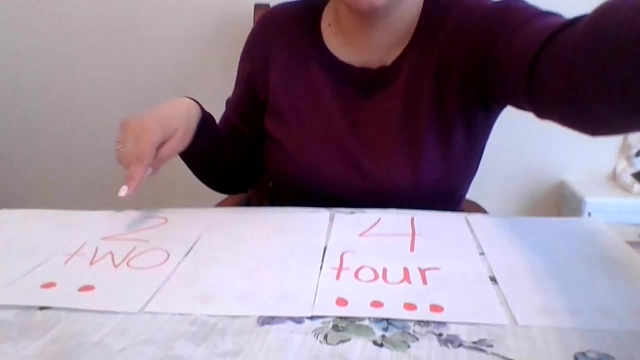 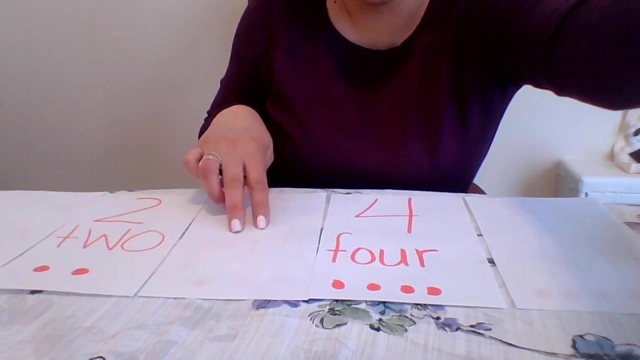 So we did 1,, 2,, 3,, 4.. Now, how's another way that you knew this was the number 4?? Yes, because you already knew this was the number 2, right, So 2,, 3,, 4.. 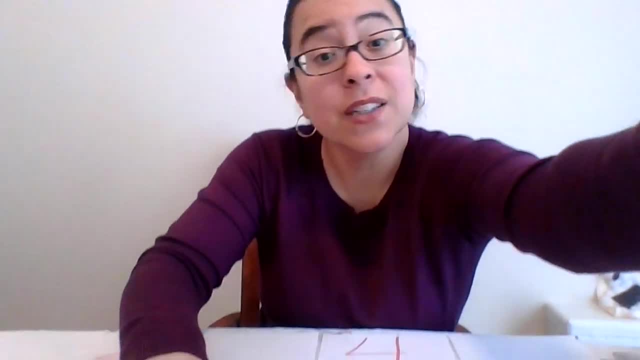 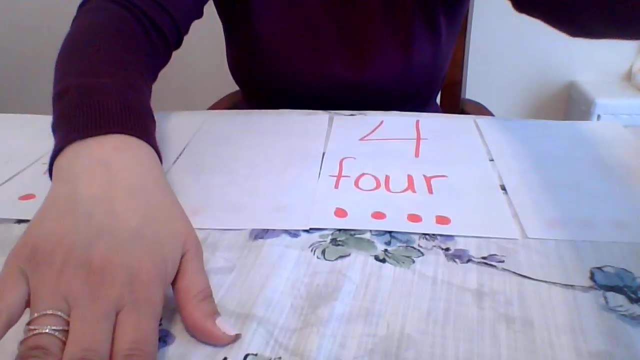 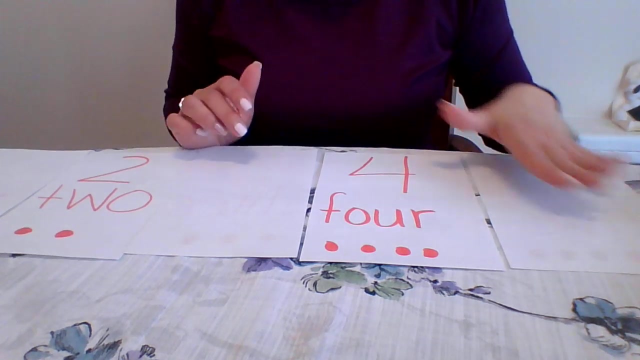 Anyone else. That's right, because the number 5 is right next to the 4. It's at the end, right? So you have 4, 5.. You counted, or 5, 4. You counted backwards, right. 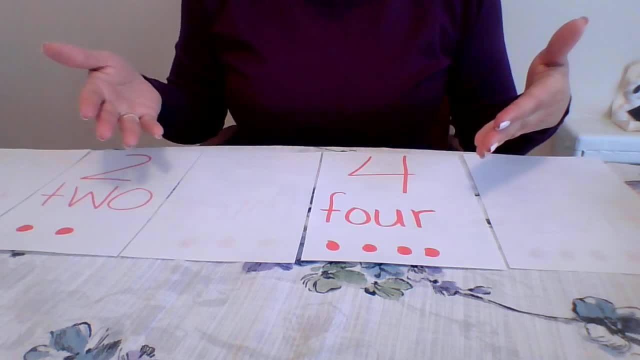 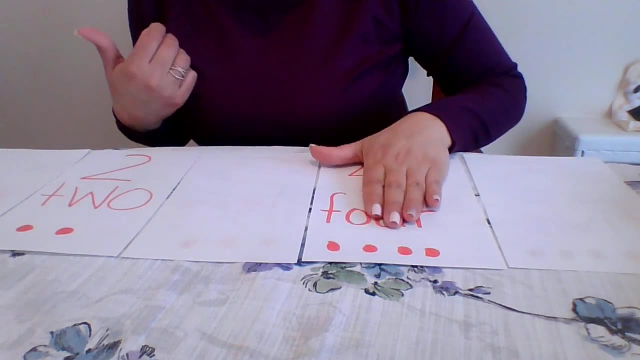 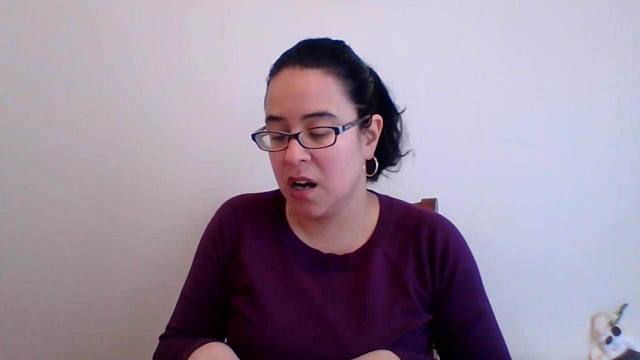 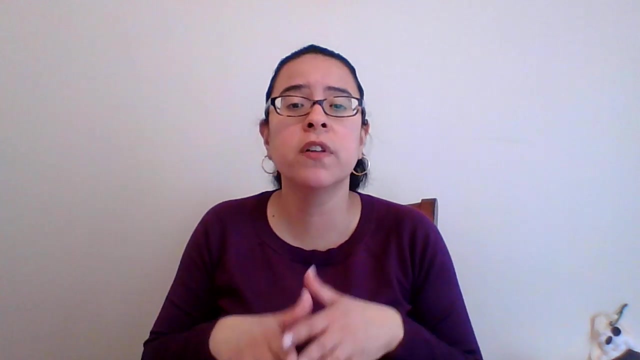 And we practiced counting backwards yesterday. right, We do, We did our backward counting, So 5, 4.. Good So, boys and girls, any time that you guess that you correctly guess a number card, you're going to leave that card facing up until all of the cards are facing up where the numbers are showing. 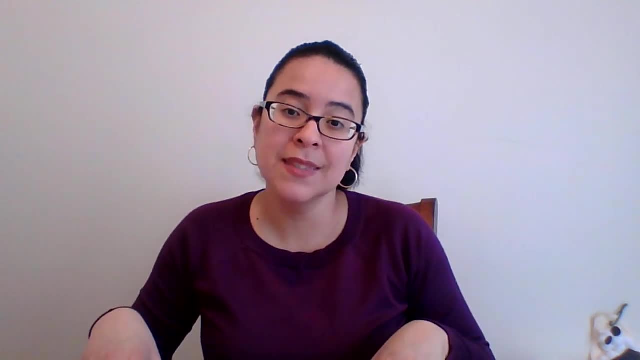 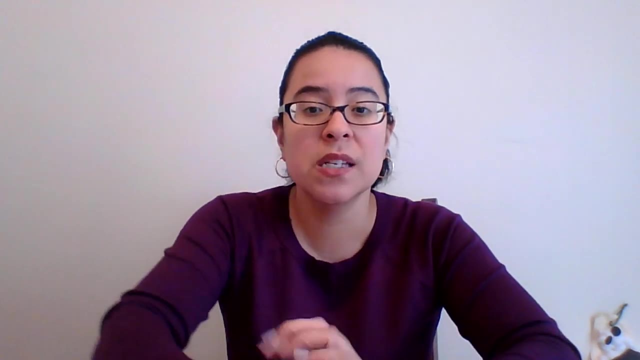 Okay, I hope you have fun doing this with maybe your older brothers and sisters Or other family members. Okay, We'll see you again later. Bye-bye.